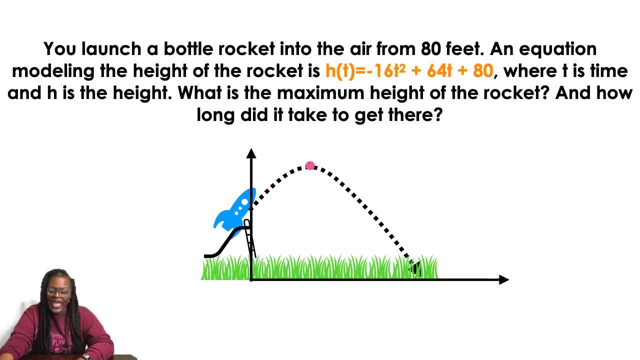 the maximum height, right? So we're gonna put a little, you know, xy-axis on the little screen. That is my maximum height and then the oh, why'd I go so quick? That represented the time, Anyway. so when maximum equals vertex, so negative b over. 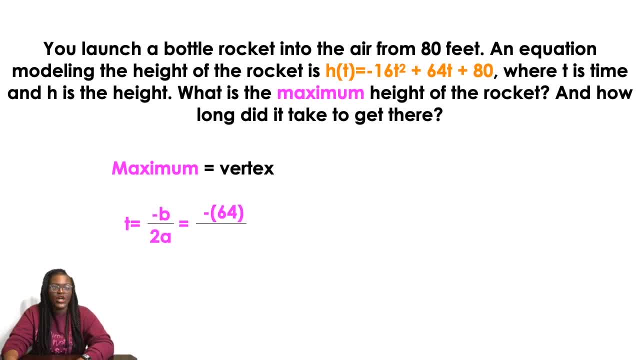 2a, right. So we're gonna plug in negative 64 over 2 times negative 16, a is 16, b is 64.. I'm gonna simplify: Negative 64 over negative 32, I'm gonna get 2.. Once I get that 2, we plug it in. Instead of t, we're gonna say 2.. We're. 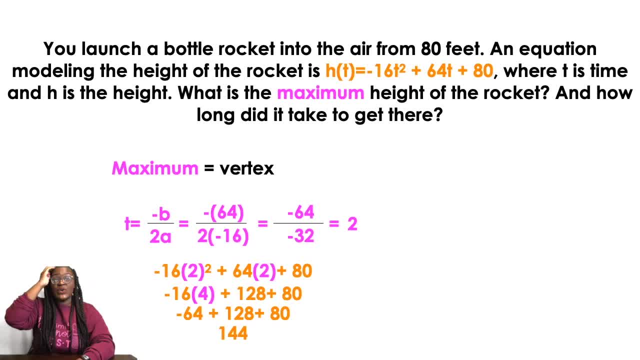 gonna simplify by using pangas and we're gonna get 144.. So this question asks us two things. It asks us what is the maximum height of the rocket and how long did it take to get there? So out of those two answers, we got a 2 and a 144.. Which one do you think represents the height? The 144,. 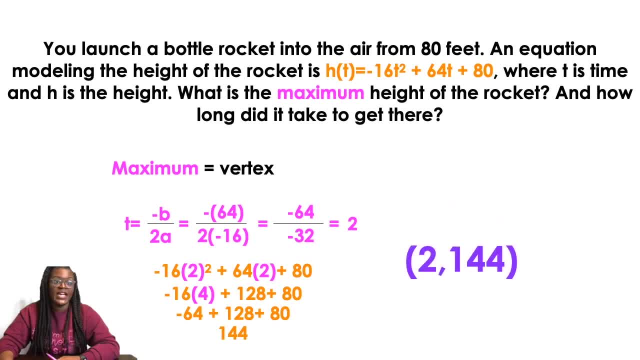 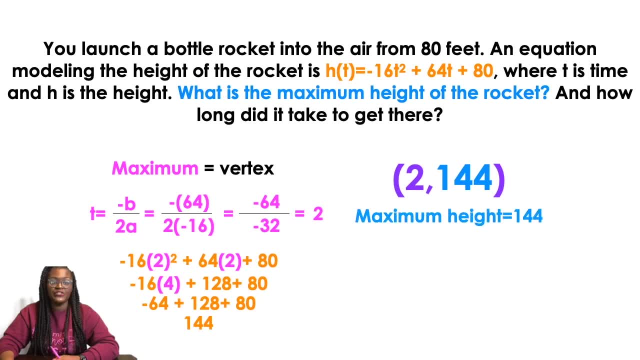 right, And which one do you think represents the time? The 2, 2 seconds. Okay, so 2 comma 144.. We will always say that the maximum height was 144 feet and it took 2 seconds to get there. That's how you do that problem. It's really just a. 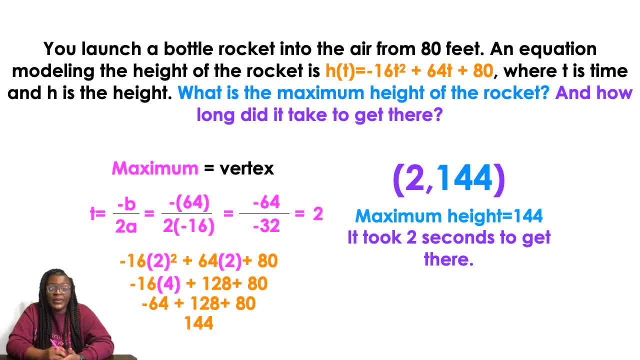 vertex problem. I know there's a lot of words going on here, but that's it in a nutshell: Find the vertex, interpret it. The x-value, the 2, is the time because, remember, on the x-axis, that's what we. 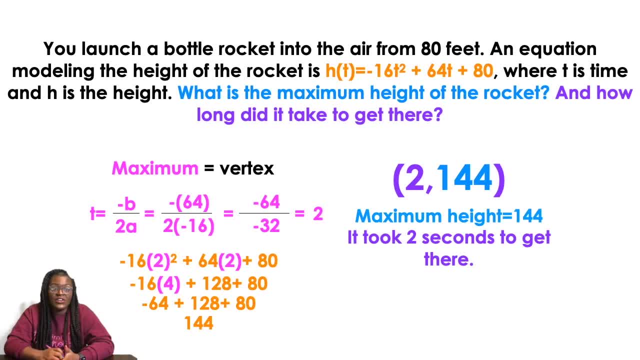 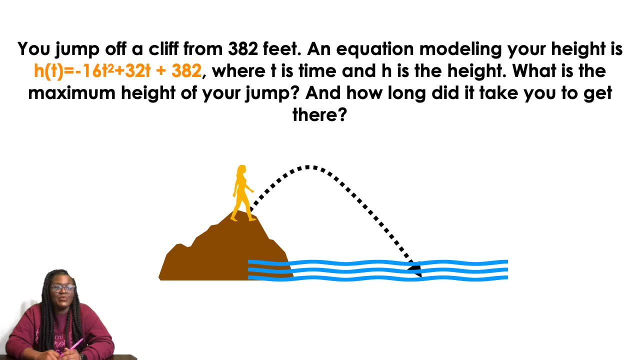 represent the time, And then the other is the is gonna be your, your height. okay, All right. Second example: you jump off a cliff from 382 feet. An equation modeling your height is: h of t equals negative 16 t squared. 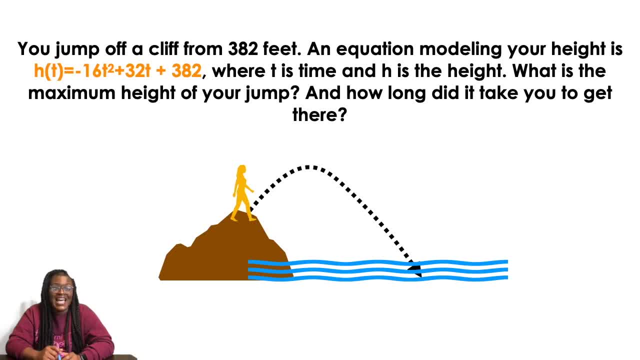 plus 32t plus 382, where t is time and h is height. What is the maximum height of your jump and how long did it take you to get that high? So look at our wonderful picture. You want your little clip? Look at me drawing drawing. This is we. 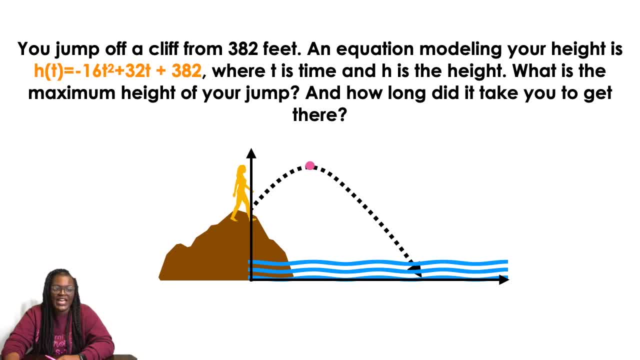 have an x-axis and a y-axis. The y-axis is vertical, the x-axis is horizontal. So that point at the top, that's our maximum height. That's what we're trying to find out. That is a vertex, And then the x-axis represents my time.